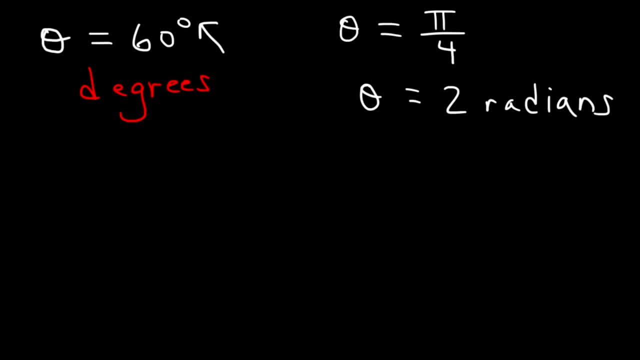 that is in radians. So this is 2 radians. So anytime you see a number without this little circle, it's radians. Now what is a radian exactly? What's the definition of a radian? A radian is basically the measure of the central angle of a circle where the arc length is equal. 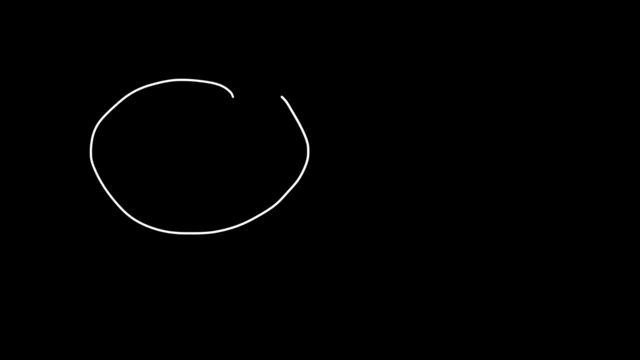 to the radius of the circle. So let's draw a circle. Okay, that is a terrible circle. Let's do that one more time. So let's say: this is the center of the circle. The radius is the distance between the center of the circle and any point on the circle. Now let's say if we draw the length of the radius, 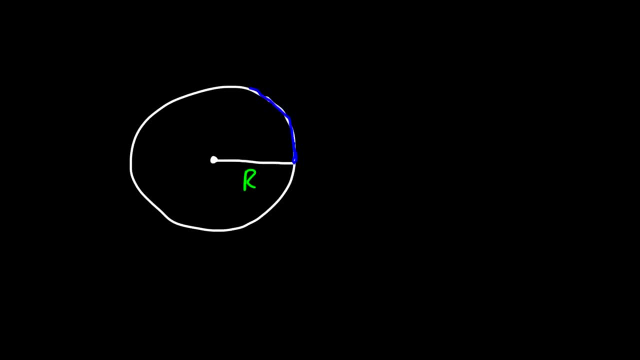 but as an arc. Let's say that distance is also arc. If we connect the center to the edge of that point, then that's also the radius. So whenever you have a situation like this where the arc length is equal to r, and it's the same, 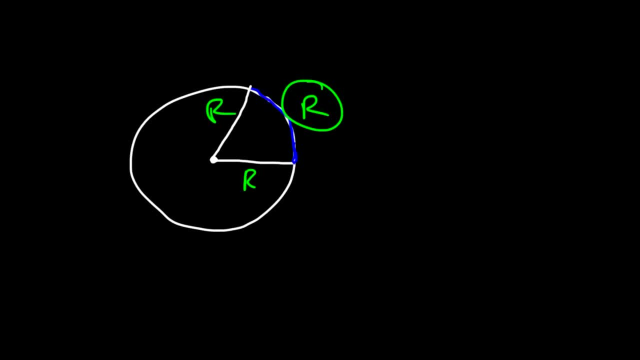 as the radius of the circle, then the angle that forms is 1 radian. So this angle is 1 radian. So that's the definition of a radian. A radian is the angle that occurs whenever the arc length iscular is the distance between the central angle and radius of the circle. In fact, if 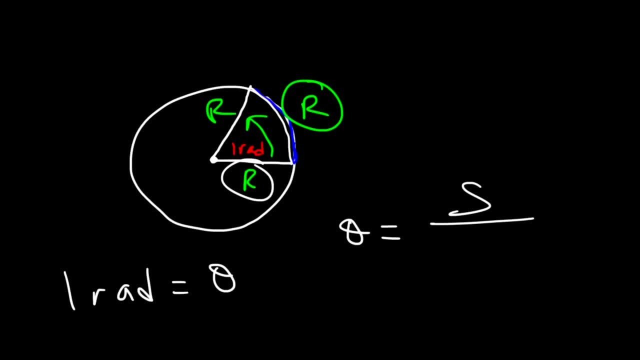 you want to find the angle, theta, you can divide the arc length, which is known as S, by the radius, and that will give you the angle in radians. So keep this in mind. Let's say: this is R, and this is R And here's S, the arc length. So if we need to find the angle, 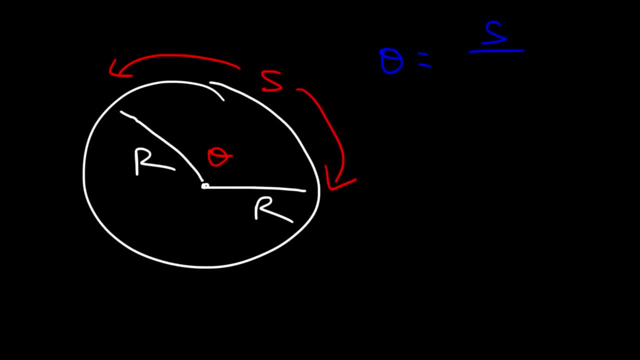 theta simply divide arc length by the radius. So let's say, if we have a circle and let's say the arc length is 12 centimeters, So that's the distance between these two points. Let's call it point A and point B And let's say point C is the center of the circle. 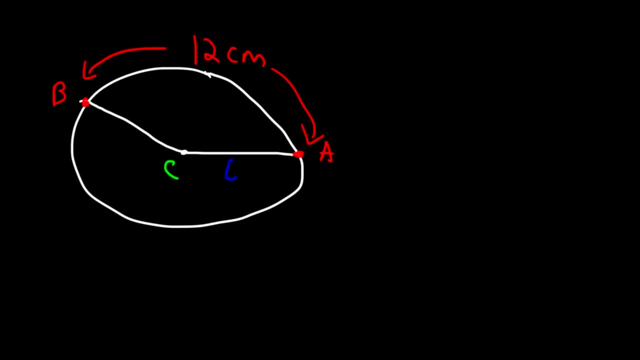 Now let's say that the radius of the circle is 6 centimeters, So that's the distance between the center and a point on the circle. What is the angle? theta in radians? What is the angle? So to find the angle, it's the arc length divided by the 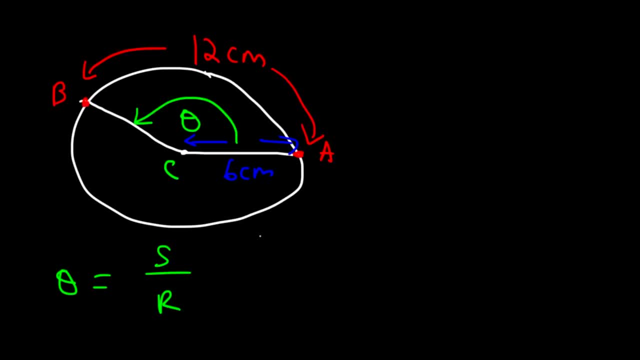 radius. So it's 12 centimeters divided by 6 centimeters, And so this will give you 2, or 2 radians. Personally, I like to think of the radius as being the left per unit radian. I think of it as being 6 centimeters per radian, And that way you can see how the unit centimeters. 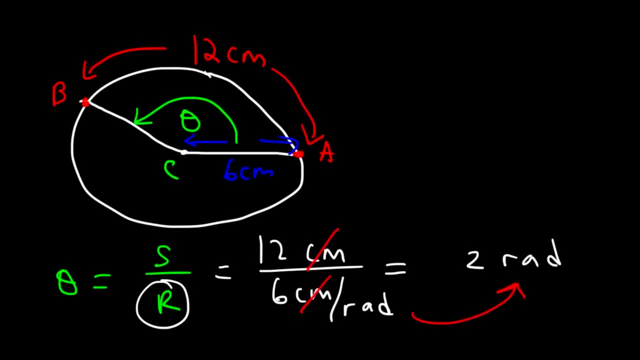 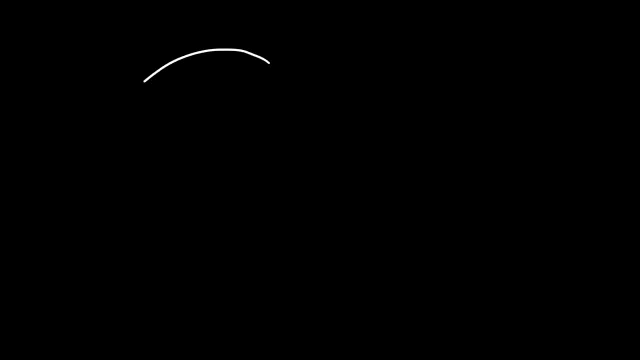 will cancel And in the end you should get radians. So that's how you can find the angle. Let's work on another example. So let's say the radius is 4 inches And let's say the arc length S. let's say S is equal to 16 inches. Calculate the angle. 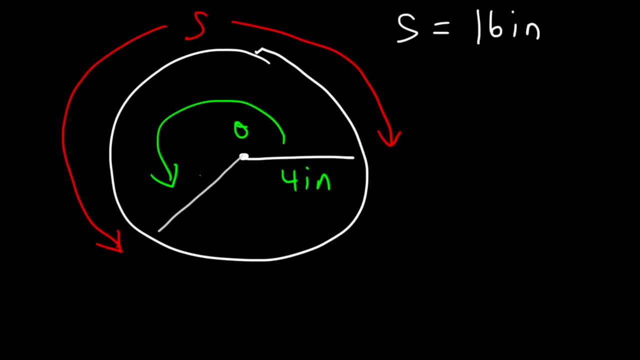 theta as indicated in the drawing. So the angle theta is going to be S divided by R, So in this case it's 16 inches divided by 4 inches. So the angle theta is going to be 16 inches divided by 4 inches, So in this case it's 16 inches divided by 4 inches. 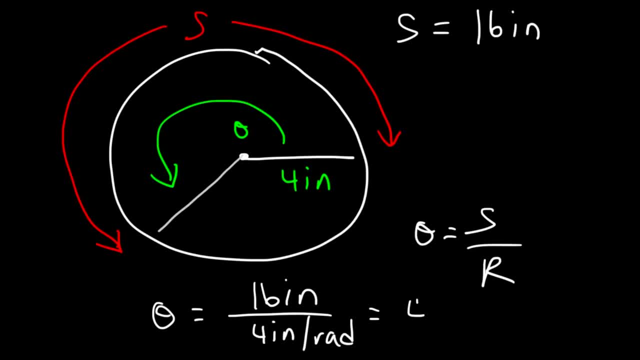 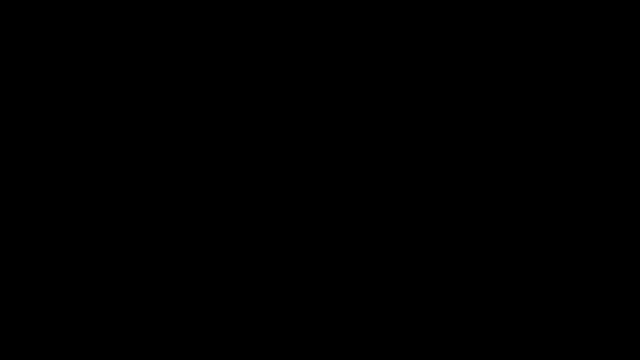 So this will give you 4 radians. So now you know how to calculate the angle in radians. if you're given the arc length and the radius, Now let's talk about how to convert angles from degrees to radians. So what you need to know is that let's say: if you have a circle, 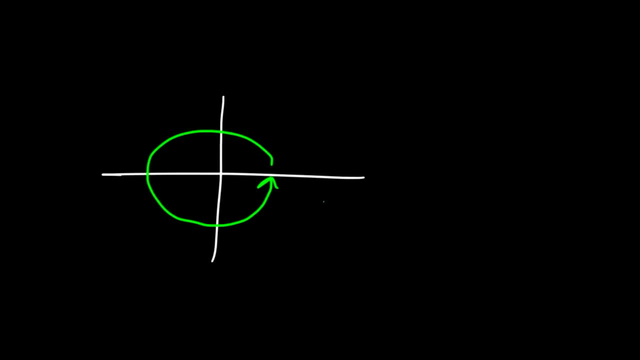 One full revolution of a circle is equal to 360 degrees, And that's equal to 360 degrees, And that's equal to 360 degrees. Now, if 360 degrees is equal to 2 pi radians, and if we divide both sides by 2, we can see. 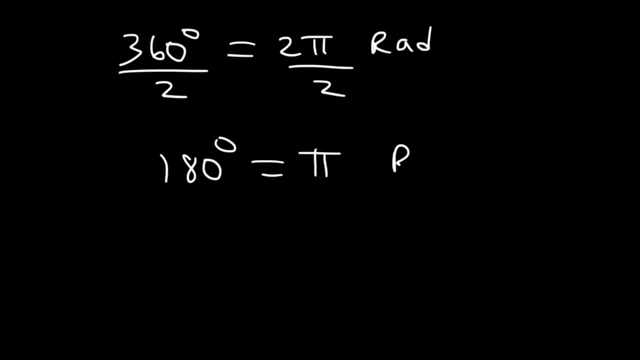 that 180 degrees is equal to pi radians And this is the conversion factor that you want to use to convert from degrees to radians. So let's say, if we have the angle 60 degrees and we want to convert it to radians, Here's what we need to do: Take your angle and then. 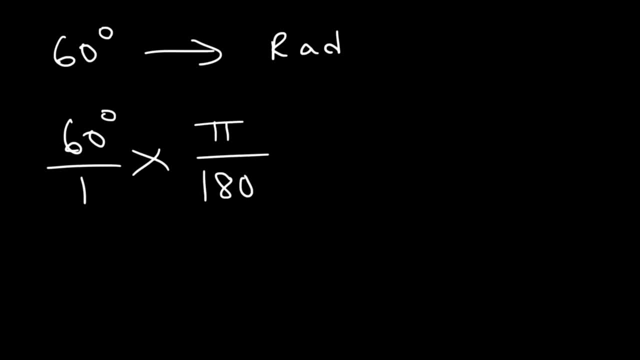 multiply it by pi divided by 180.. You want the unit degrees to cancel. So what's 60 divided by 80?? For one thing, we can get rid of a 0, so it becomes 6 over 18.. So we have 6 pi over 18, but we can write 18 as 6 times 3. And we can cancel a 6.. 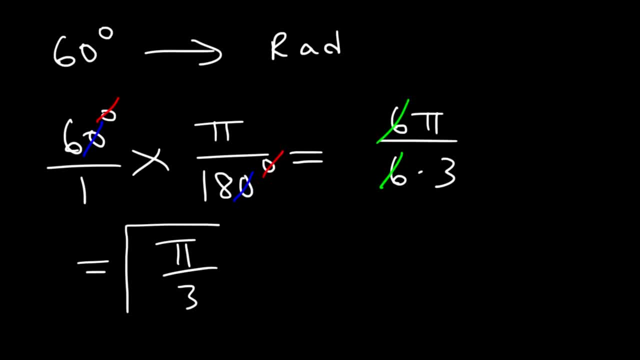 So therefore, the final answer is pi over 3.. So 60 degrees is equal to pi over 3 radians, And that's okay. You can make another example: Convert 150 degrees into radians. Feel free to pause the video and try this problem. 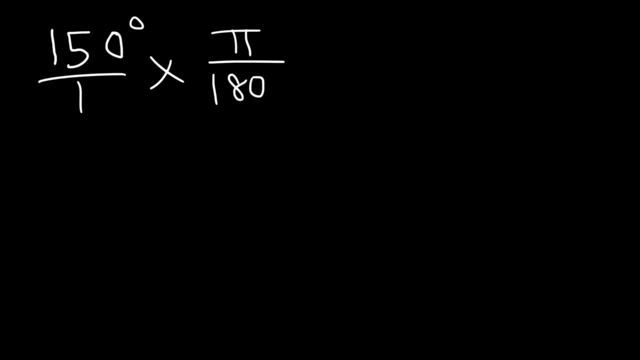 So, just like before, we're going to multiply by pi divided by 180.. So let's begin by getting rid of a 0.. So now we have 15 pi divided by 18.. 15 is 5 times 3.. 18 is 6 times 3.. So we 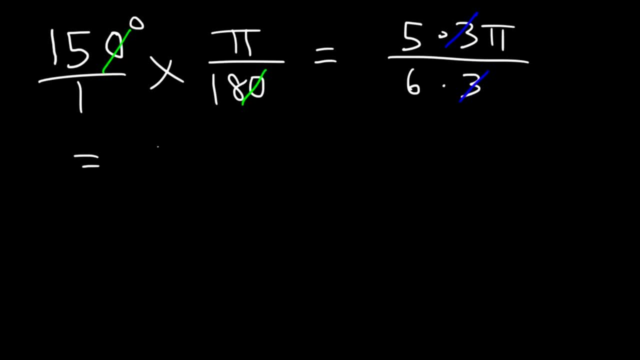 We can get rid of a 3, so therefore, the final answer is 5 pi divided by 6.. Try these two examples: Convert negative 225 degrees into radians and also negative 30. So I'm going to start with negative 30. 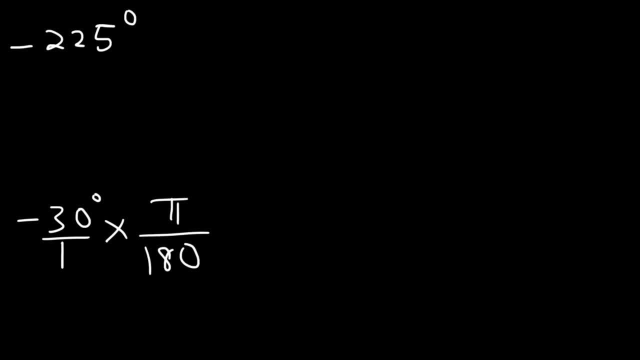 Let's multiply that by pi, divided by 180.. So once again we can get rid of a 0.. So this is going to be negative: 3, pi and 18. I'm going to write it as 6 times 3.. So we can cancel a 3.. 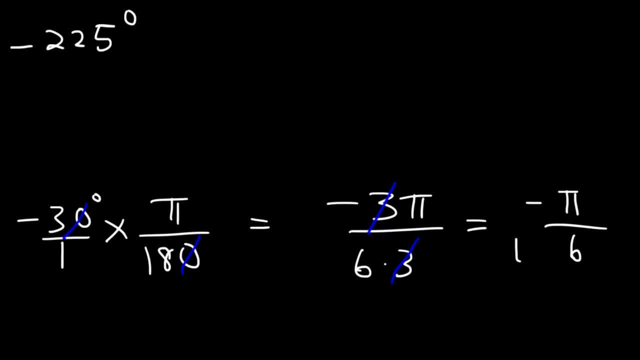 So the final answer is going to be negative pi divided by 6.. That's equal to negative 30 degrees. Now, in this example, let's multiply negative 225 degrees by pi divided by 180.. Now it's helpful to know that 225 is 45.. 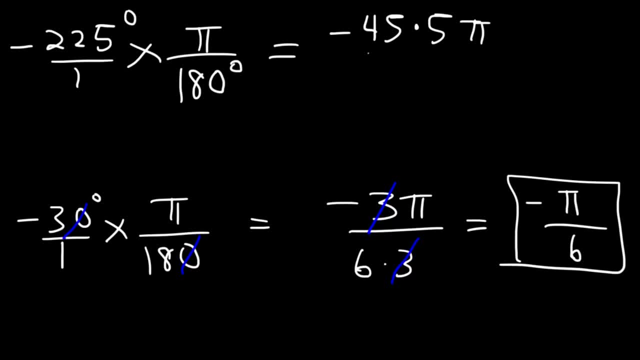 Okay, Okay, Now we're going to consider negative 35 times 4.. So now we can cancel 45, which will give us a final answer of negative 5 pi divided by 4.. So now you know how to convert angles from degrees to radians, and that's all you need. 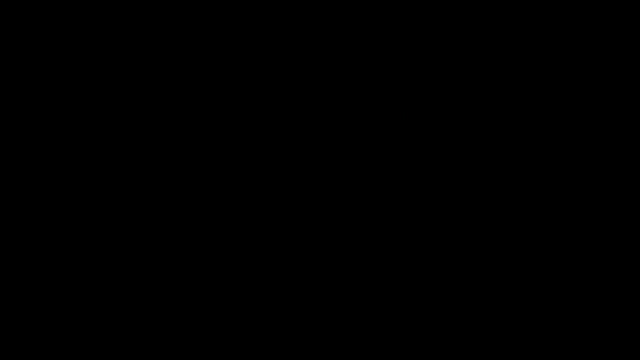 to do? Just multiply by pi over 180.. Now what about converting radians into degrees? So let's say, if we have 2 pi over 3 radians, What should we do to convert this angle into degrees? Well, this time, instead of multiplying by pi over 180, we're going to multiply by 180. 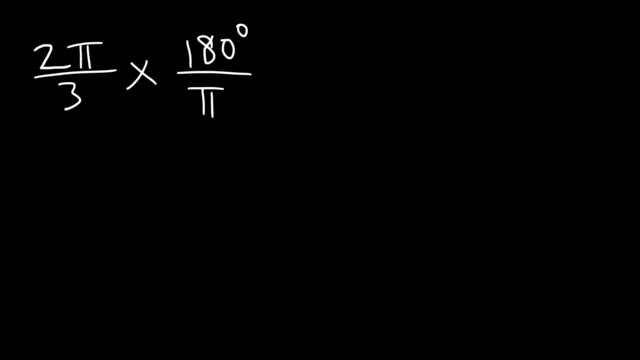 divided by pi. We need to flip it Now. you want to write it in such a way that the pi letters cancel, So this is going to be 2 times 180 divided by 3.. Now 180 is 60 times 3.. 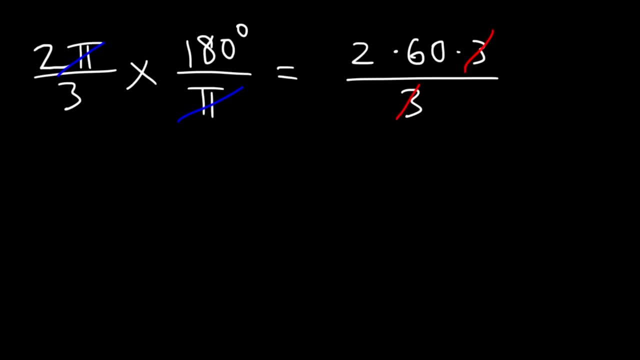 So we can get rid of 3.. And so we're left with 2 times 60,, which is 120 degrees. And so that's the answer. Let's try some more examples. Try this one: Convert 11 pi over 6 into degrees. 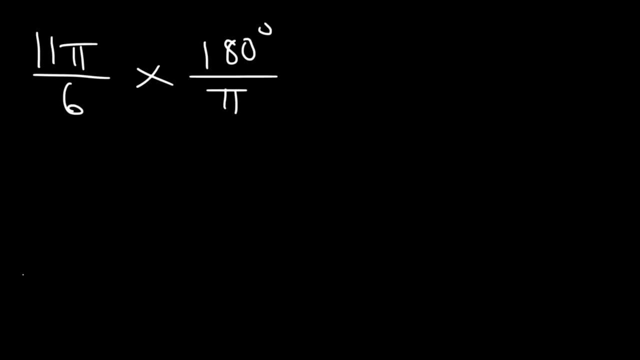 So once again, let's multiply by 180 divided by pi. Let's cancel pi. Now we can write 180 as 30 times 6.. So let's get rid of 6.. So we just got to multiply 11 times 30.. 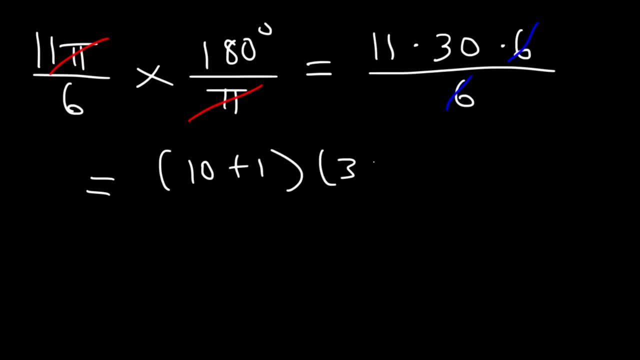 11 is basically 10 plus 1.. And if we distribute 30 to it, 30 times 10 is 300, and 30 times 1 is 30. So our final answer is 330 degrees. Okay, Here are some examples that you can try. 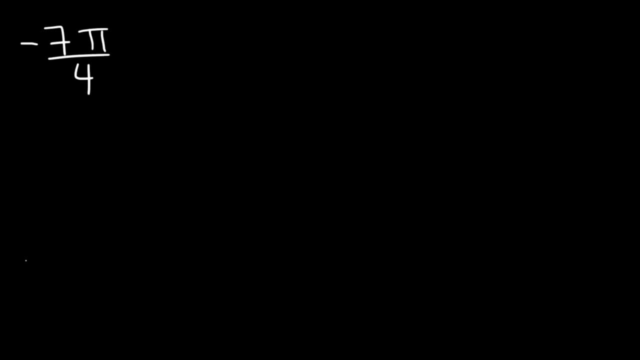 Convert negative 7 pi over 4 into degrees, and also negative 3 pi over 2.. So I'm going to start with this one. Let's multiply by 180. divided by pi, 180 is the same as 90 times 2.. 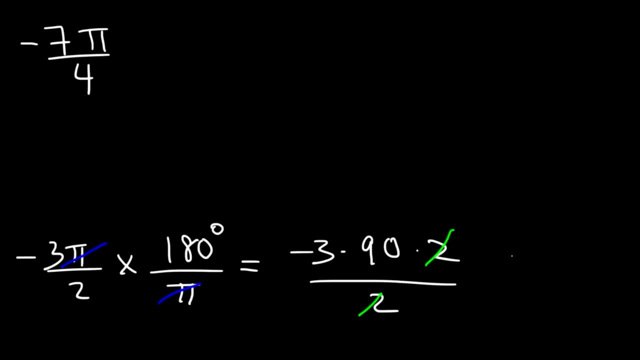 So we can get rid of 2.. And 3 times 90 is 270.. So the final answer is negative 2.. Negative 270 degrees. Now what about negative 7 pi over 4?? Well, let's do the same thing. 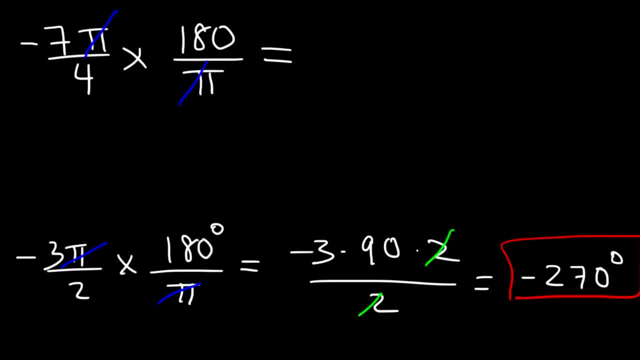 Let's multiply by 180 over pi and cancel pi. Now, keep in mind, 180 is 45 times 4.. So we can cancel 4.. So now we need to multiply 45 times 7.. So that's the same as 7 times 40 plus 5.. 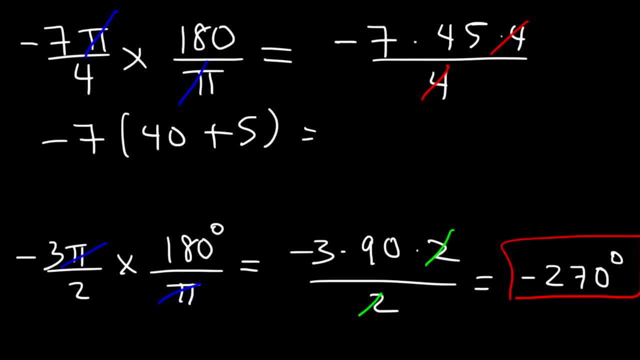 Okay Now 7 times 40.. If 7 times 4 is 28,. 7 times 40 is 280.. 7 times 5 is 35.. If we add 280 and 35, this is going to be 315.. 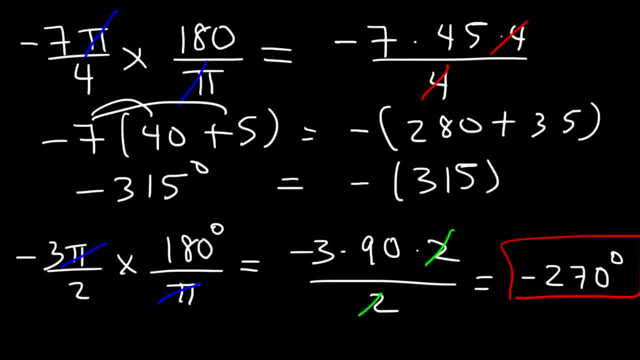 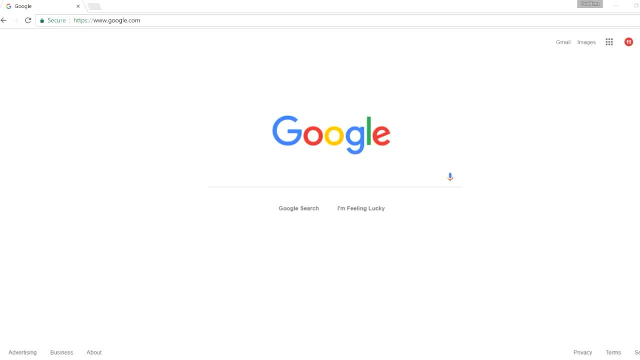 So the final answer is negative 315 degrees. Now for those of you who want access to my complete online trigonometry course, It's a very easy one. It's called Euler's law of equation. Here's where you can find it. 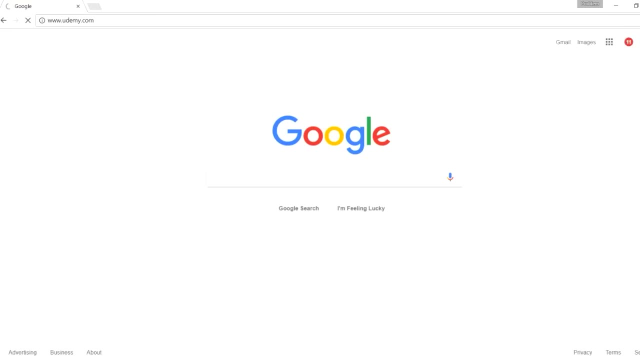 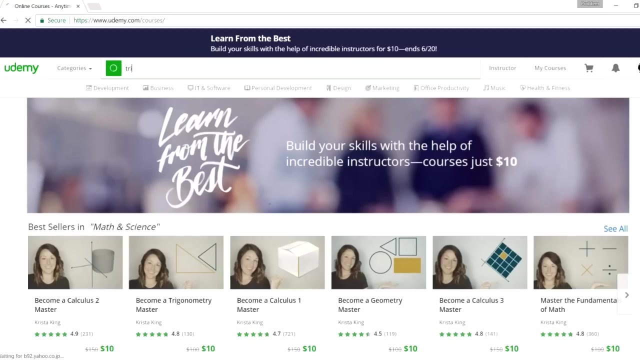 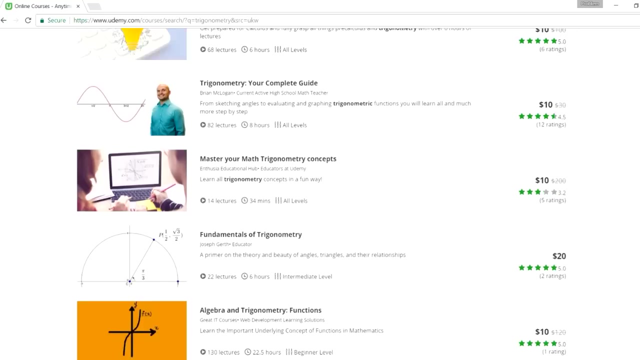 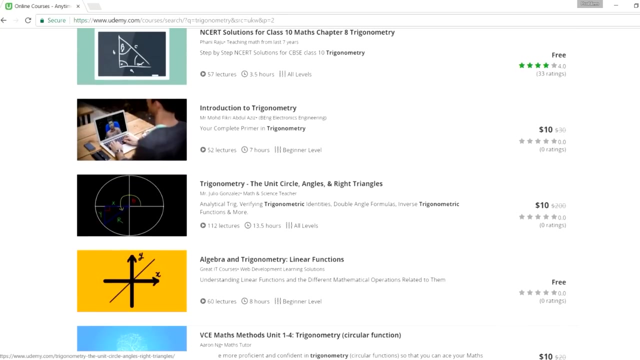 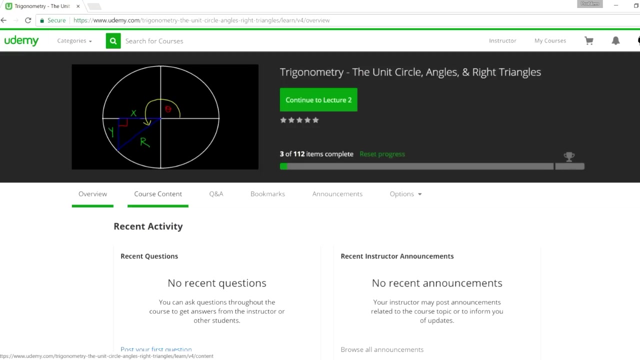 Go to udemycom and then in the search box you can just search for trigonometry And you can see. my course is basically the one with the black background, And then here is it. I'm still adding more lectures, but here's what I have so far. 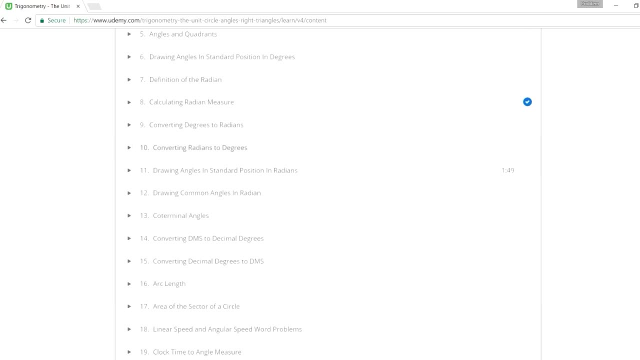 Introduction to angles: drawn angles, converting degrees into radians. linear speed, angular speed problems, arc length, information on the unit circle. how to evaluate trigonometric functions using the unicircle, right triangle trigonometry- things like SOHCAHTOA. 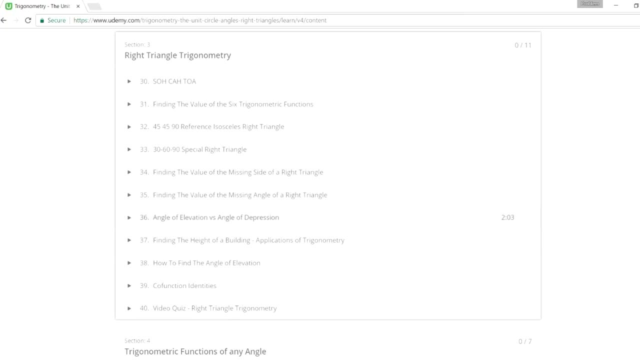 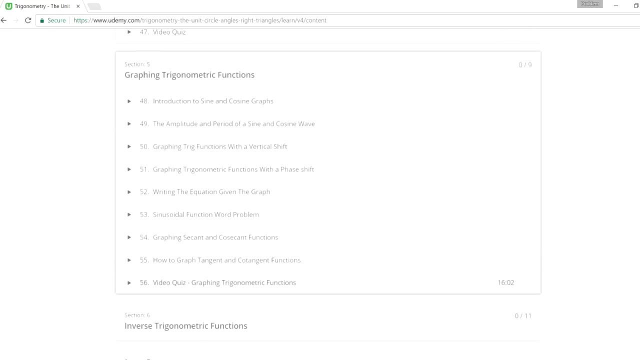 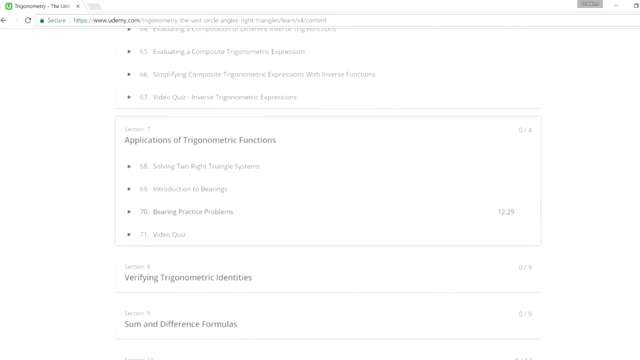 Even you can have video quizzes as well, solving word problems like angle of elevation problems. And then you have the next section: graphing sine cosine functions, secant tangent, inverse trig functions- pretty much all the common stuff that you'll see in a typical trigonometry course. 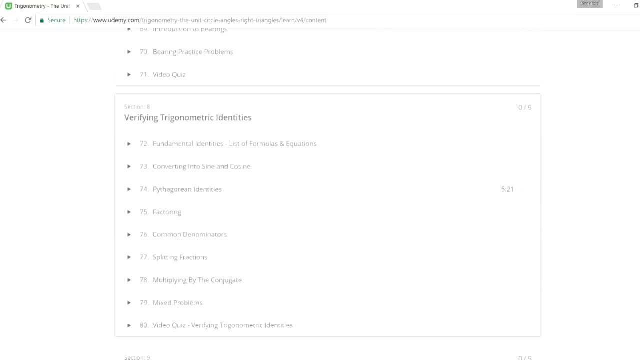 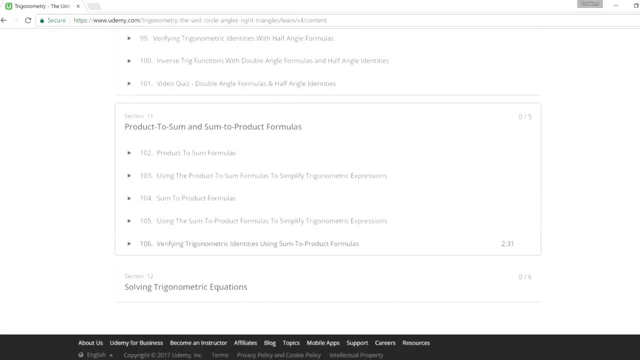 even solving Behrens, verifying trigonometric identities, some indifference formulas, double angle, half angle and some other things too, And, as I mentioned before, I'm gonna add some other things as well, So feel free to check it out when you get a chance. 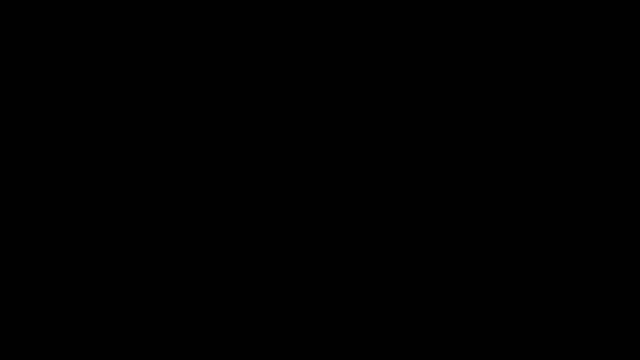 and let's continue back to the video. Now you need to be able to draw angles in standard positions. if it's given to you in radians, We've covered degrees already. So let's say, if we have the angle pi over four, How can we graph it in standard position? 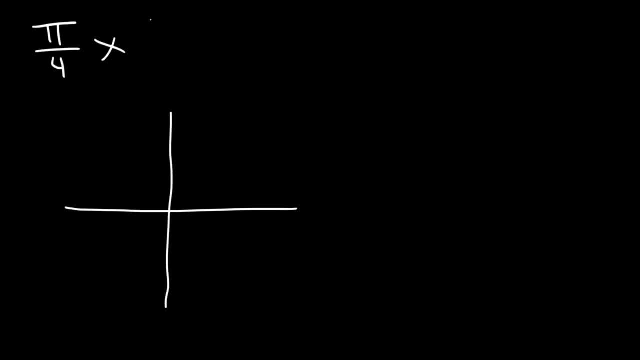 Well, for one thing, it might be helpful to convert this into degrees: 180 divided by four is 45 degrees, And you know 45 is between zero and 90. So we're gonna draw the ray right in the middle between those two. 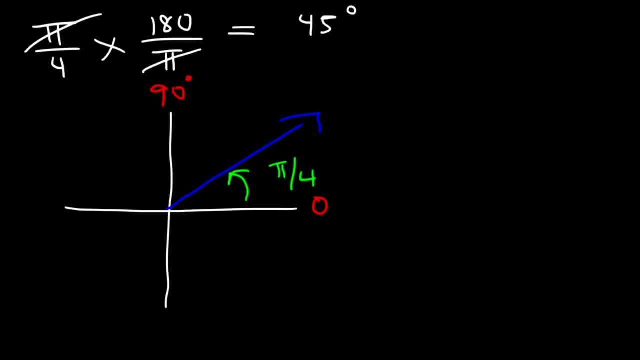 So, therefore, this is how you graph the angle: pi over four. Let's try another example: Seven, pi over six. Where should we graph it? Well, let's begin by converting it into degrees: 180 is 30 times 60.. 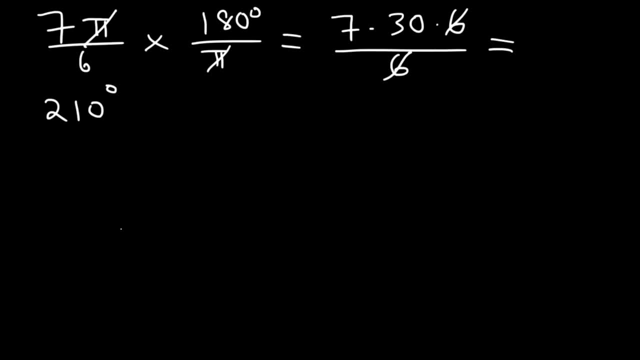 And seven times 30 is 210.. Now 210 is between 180 and 60. Now 210 is between 180 and 60. And 270, but it's closer to 180.. So it's right there. Therefore, this angle is seven pi divided by six. 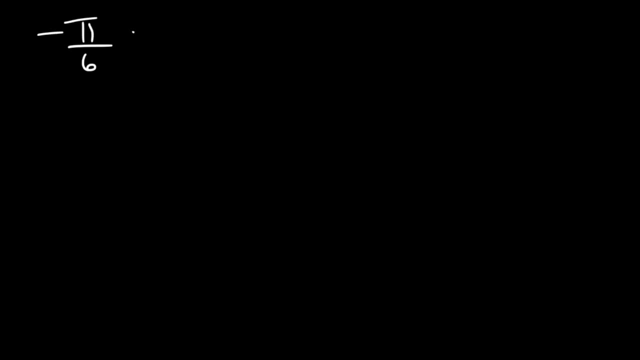 Try this one Negative pi over six. So let's convert it to degrees first. 180 divided by six is 30. So this is zero and this is negative 90. So negative 30 should be in this region In quadrant four. 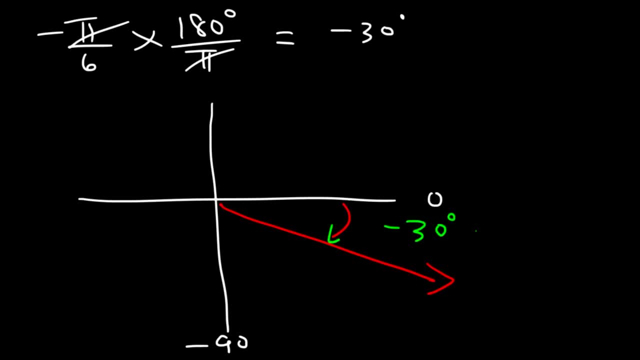 So this is negative 30 degrees. Now let's talk about some common angles that you need to know in radians and their locations. Let's start with pi over four. So pi over four is located in quadrant one. It's between zero and 90.. 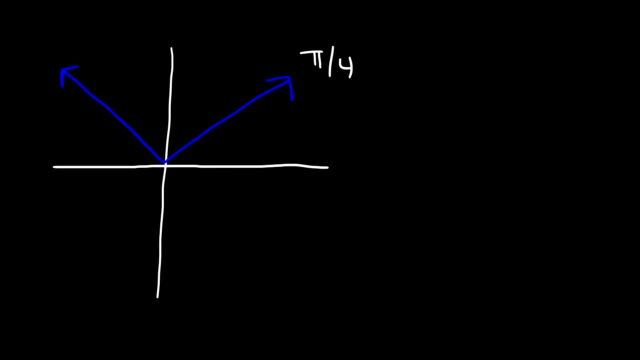 The next one that's similar to it, that you need to know, is three pi over four. Three pi over four is 135.. Pi over four is 45. So 45 times three is 135.. In quadrant three, the next angle is five pi over four. 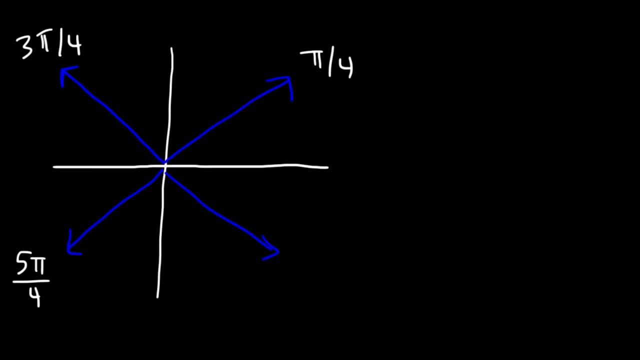 which is 225.. And quadrant four has the angle seven pi over four. Seven times 45 is 315.. Now this angle here is two pi over four. Two pi over four, it reduces to pi over two. And whenever you see pi, remember pi is equal to 180. 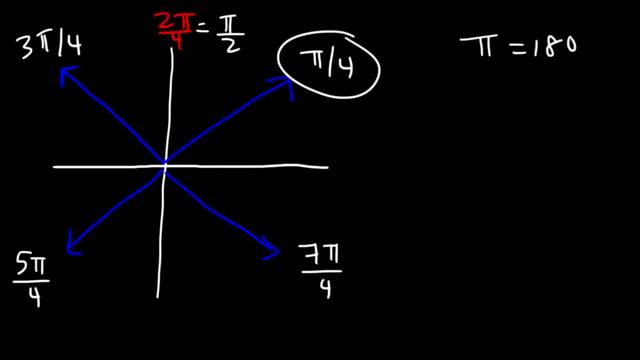 So 180 divided by four is 45.. So that's how you can remember: pi over four is 45.. Three pi over four, 45 times three, that's 135.. Five pi over four, five times 45,, that's 225,. 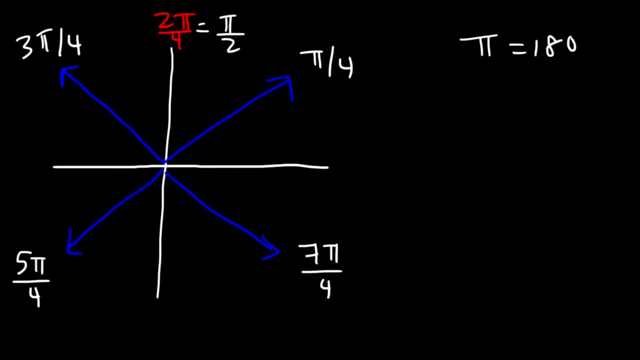 which is in quadrant five. Now the next one: four pi over four, that's 225.. And four pi over four reduces to pi, And pi is 180.. Here we have six pi over four, which reduces to three pi over two. 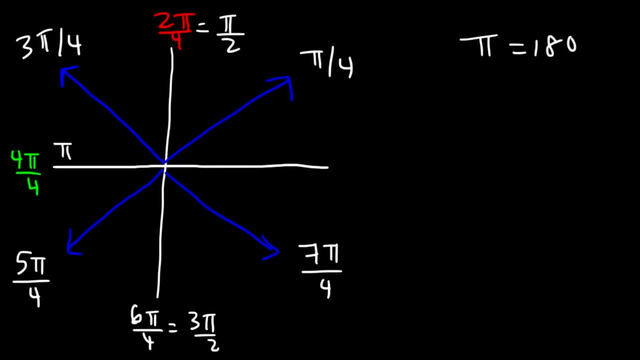 So you won't hear two pi over four, six pi over four, four pi over four, because they're reducible fractions, Just know where they're located, and that the fact that they're gonna reduce to pi over two, three pi over two or pi, 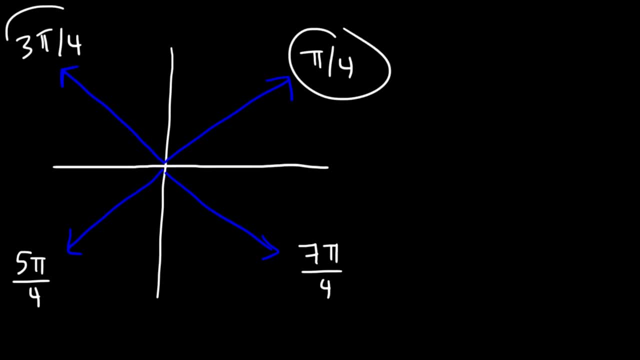 But these are the main ones you need to know: Pi over four, Three pi over four, Five pi over four And seven pi over four. Now the next angles you need to be familiar with is pi over three. So pi over three is about 60 degrees. 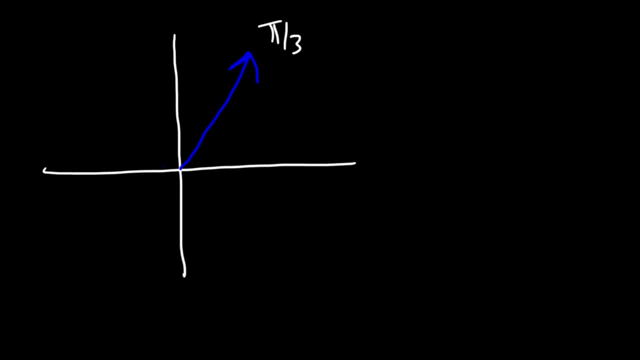 So this is one pi over three, And then two pi over three is in quadrant two, So that's about 120.. So remember, pi is 180.. So pi divided by three, 180 divided by 3, that correlates to 60. 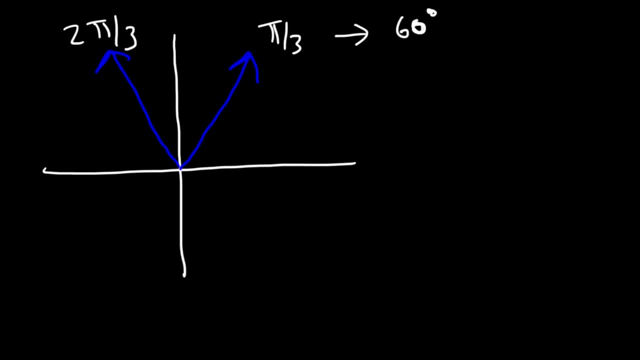 So 2 pi over 3 is 60 times 2,, which is 120.. 3 pi over 3 simplifies to pi, which is 180.. So you won't see 3 pi over 3, it'll just be pi. 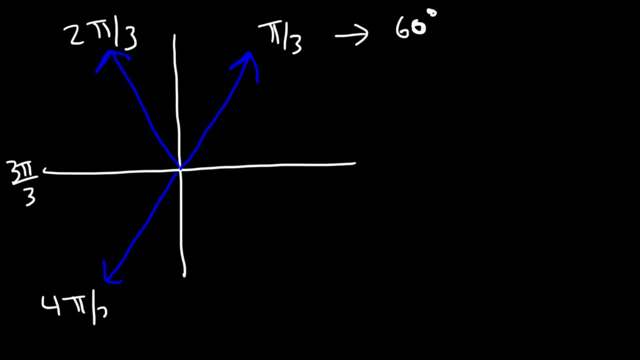 Next, you have 4 pi over 3,, which is 4 times 60,, that's 240.. And then 5 pi over 3,, that's 5 times 60, which is 300.. So, in terms of pi over 3's, those are the common ones, you'll see.